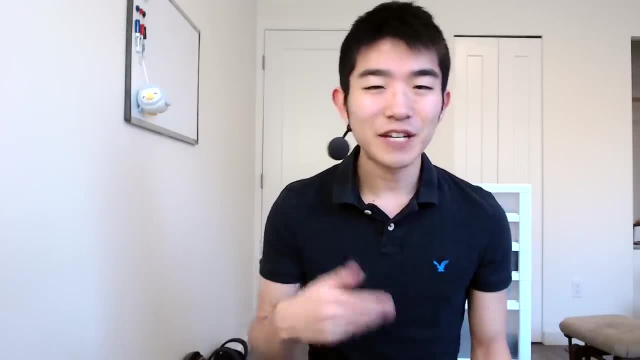 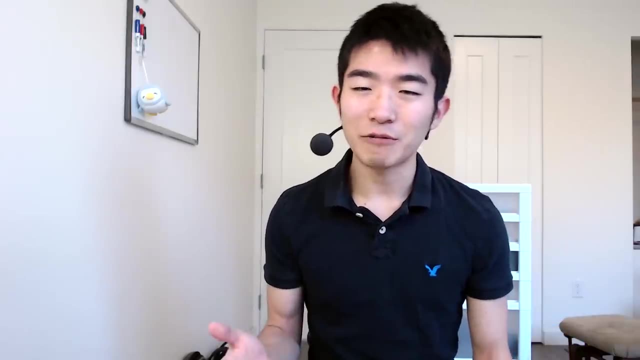 So this series is going to be good for complete beginners who've never done any programming before, as well as someone who's done some programming before, whether it's Python or any other language, but wants to learn more about Python. So in this video I'm going to go through a number 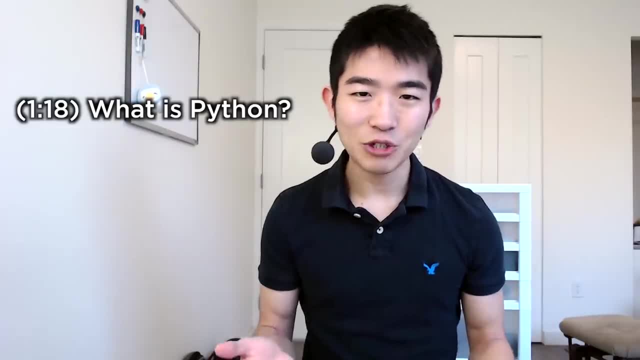 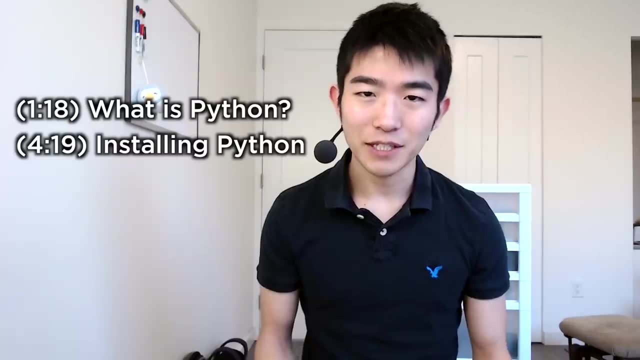 of different things. First of all, what is Python and what can you do with it? And then I'm going to explain how to install Python on your computer and then set up a development environment. We're going to use something called Jupyter Notebook throughout this series. 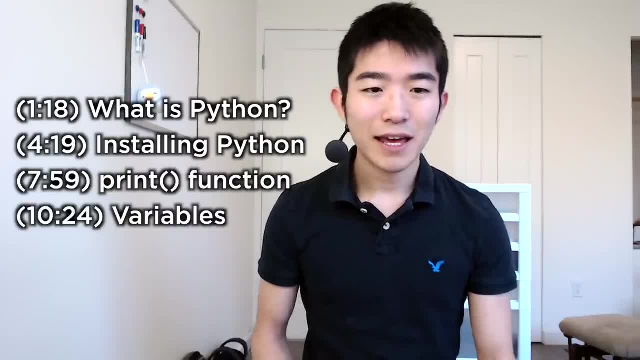 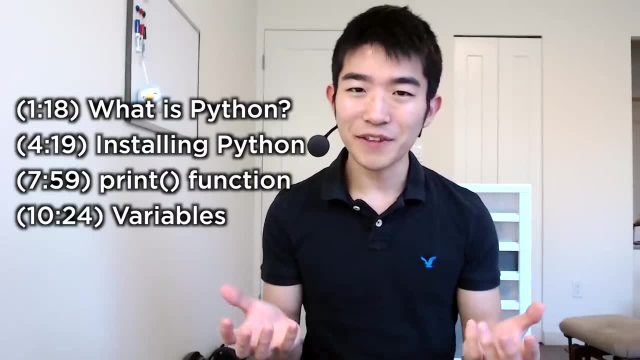 And then I'm going to explain how to use the print function and what are variables and how to use them. And by the end of this video, if you have two variables storing different things, you're going to be able to do a lot of things. So let's get started. 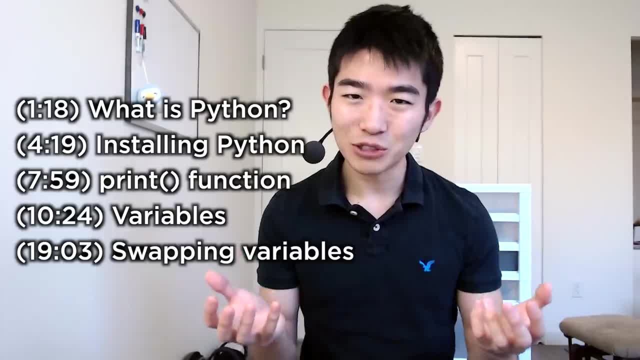 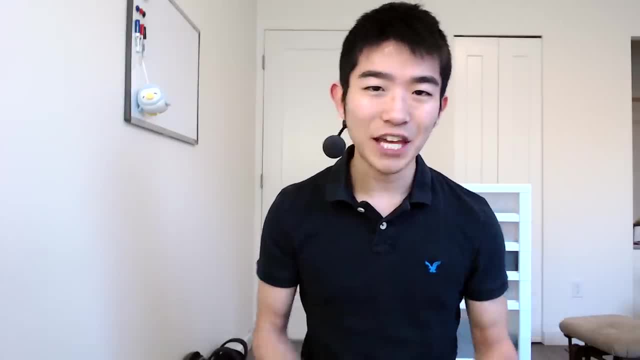 You'll be able to swap the content within those two variables with each other, And I'm going to put an outline of this video in the comment section below, so you don't have to watch the whole thing if you don't want to. Oh, and before we get started, if you want to make sure that, 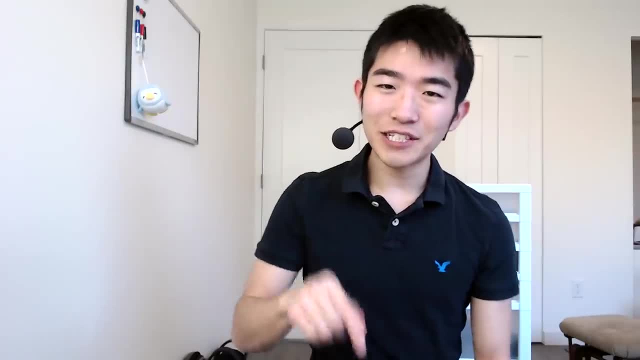 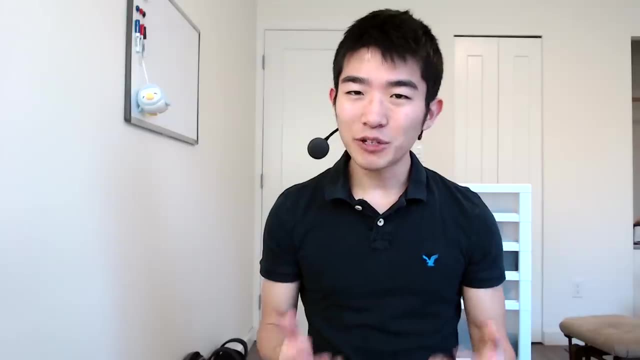 you don't miss my future tutorial videos, sign up to my newsletter, which is available in the description below. So just quickly: what is Python and what can you do with it? It's one of the most popular programming languages out there and it's used at smaller companies and it's used at 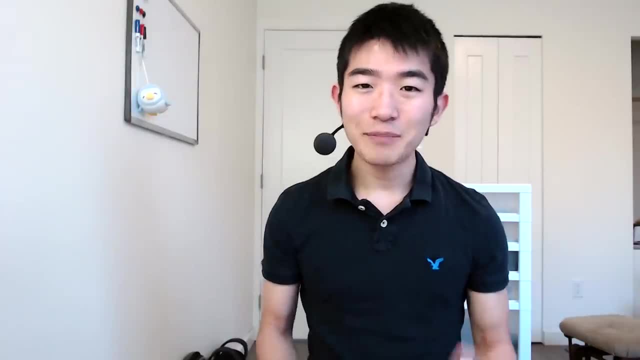 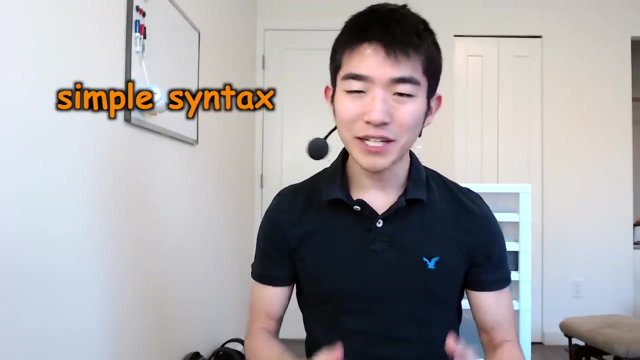 as well as larger companies including Google, And many universities use Python as the introductory programming language in their computer science courses, And one advantage of Python is that it's fairly easy to learn because it has fairly simple syntax. It's used for many different applications. 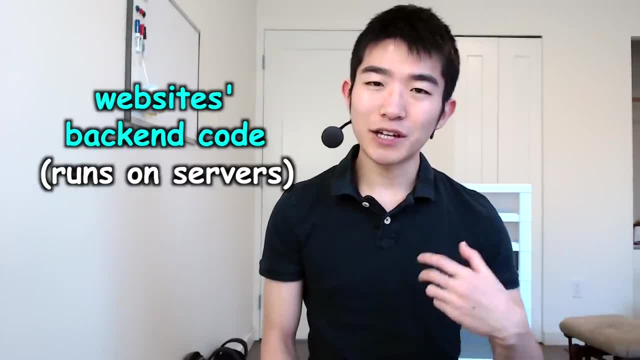 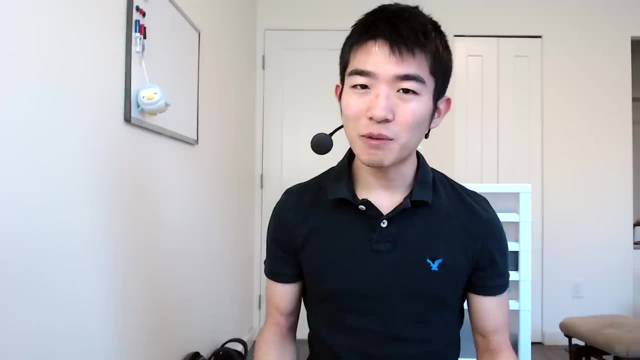 including websites' backend code, which is the code that runs on your server, as opposed to the code that runs on your device, whether it's a phone or a laptop, And it's also popular for data analysis and scientific research purposes. Okay, so let's now go ahead and install. 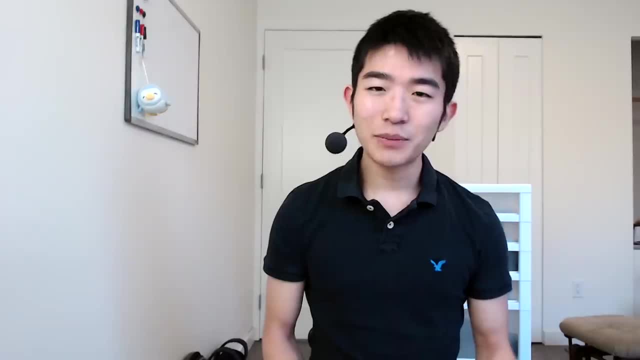 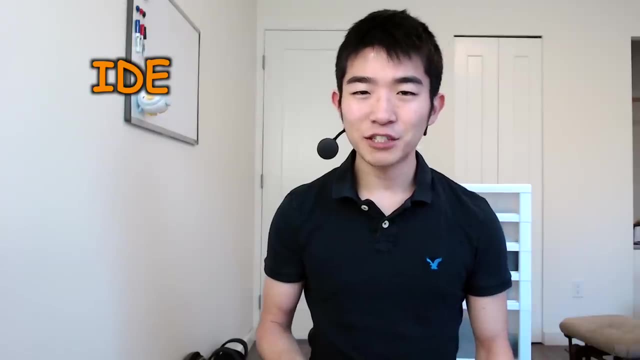 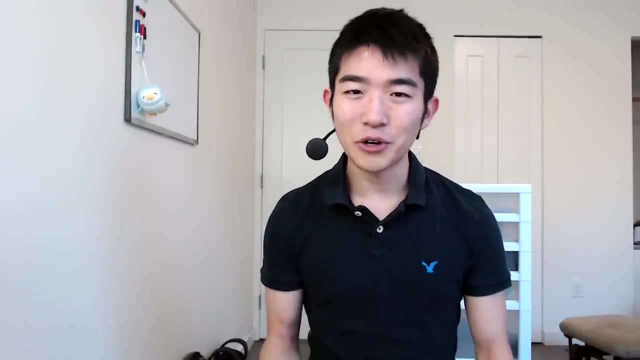 Python on your computer. Usually, when people develop a program using Python- or any other language for that matter- they usually use something called IDE, which stands for Integrated Development Environment. It's an environment that includes everything you need, pretty much, to develop a program. It has a nice text editor in which you can write your code and then the 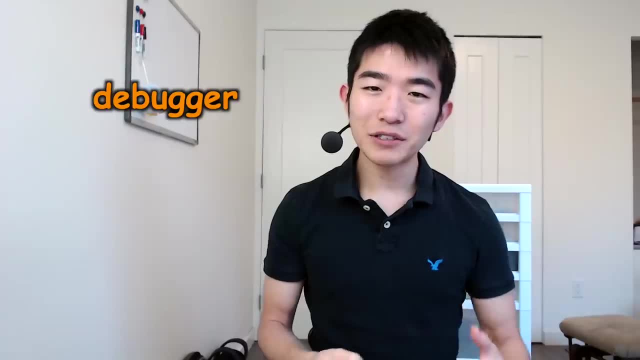 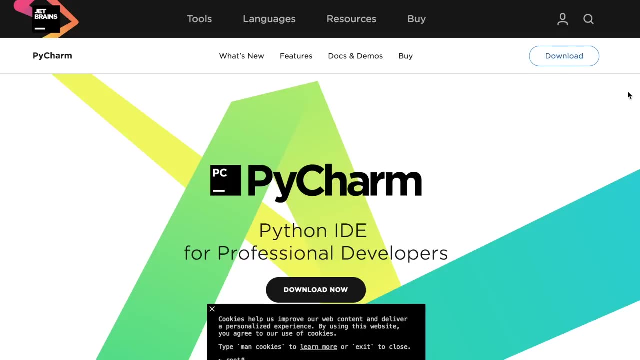 ability to run your code. So if you're using Python, you can use Python to run your code and as well as something called a debugger, which allows you to quickly get rid of all the bugs in your program. And if you want to use an IDE to follow my series, I'd personally recommend PyCharm's. 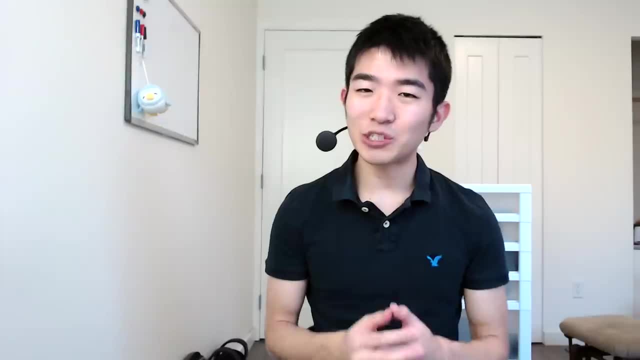 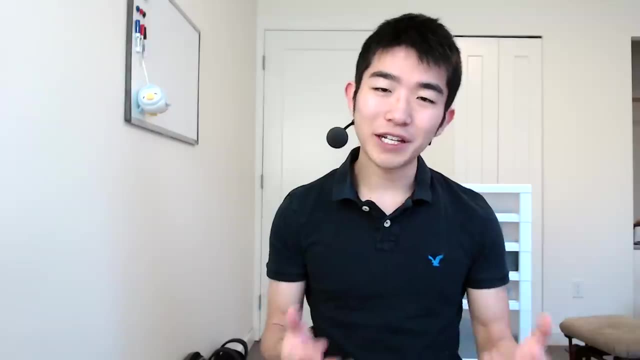 Community Edition. So in this series, instead of using a traditional IDE, I decided to use something called Jupyter Notebook. So Jupyter Notebook is an environment for writing and testing your program quickly, and it's actually popular with the scientific community and for data analysis. 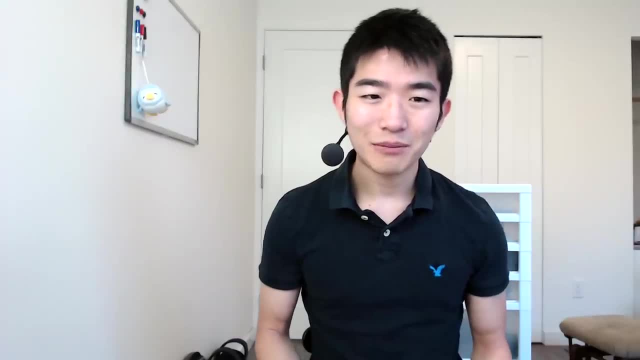 as well, But I've decided to use Jupyter Notebook throughout this series because it's very simple and easy to install Jupyter Notebook through something called Anaconda and it's fairly easy to use as well. So here's the way Jupyter Notebook works. There are two components to 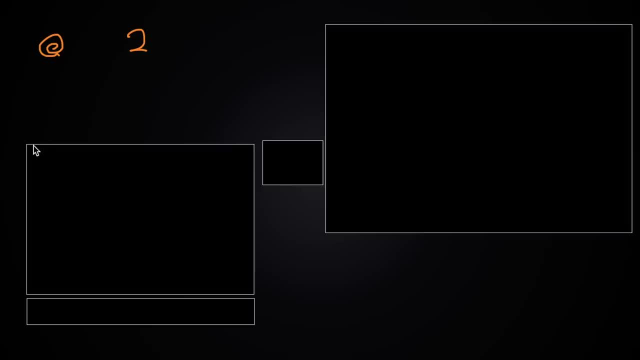 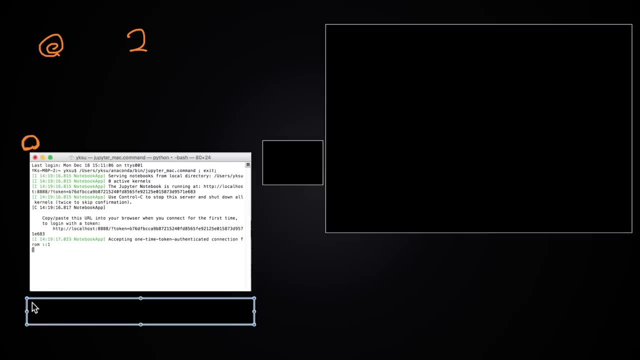 Jupyter Notebook. First of all, when you launch Jupyter Notebook on your computer, you might see a command line interface like this. This represents the Jupyter Notebook server. You can think of it like the core of Jupyter Notebook and you don't have to worry that much about how it works exactly. 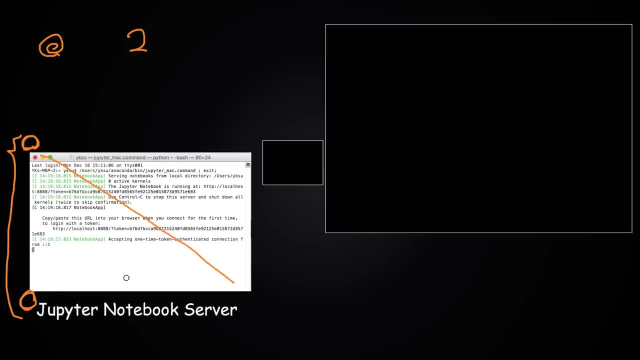 but just remember that if you close this window, maybe accidentally Jupyter Notebook might stop working, So just be careful about that. Now, when you launch Jupyter on your computer, you might also see a browser window or tab showing up, whether it's Chrome, Firefox, 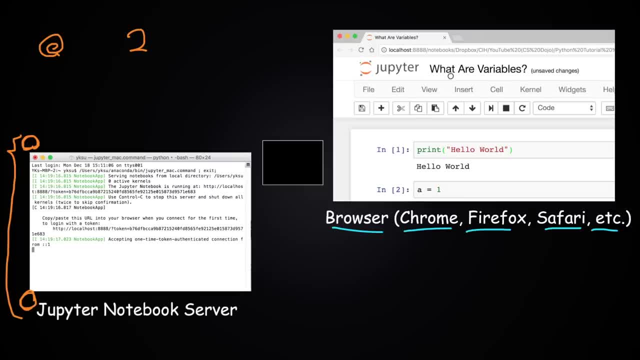 Safari or anything else, And it'll probably be at the URL logo host, column 8888 or something like that, and it'll be connected to the Jupyter Notebook server. This browser window, or tab, is basically the user interface for Jupyter Notebook and you can write and execute your code here. 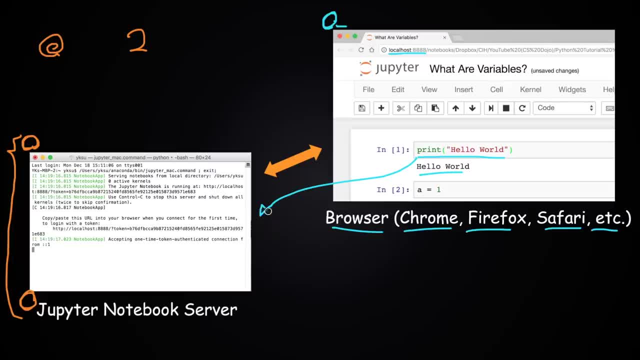 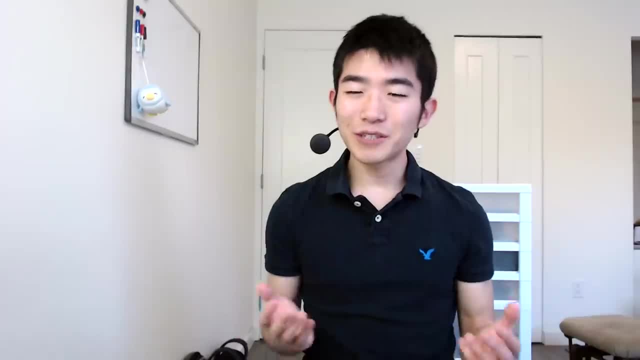 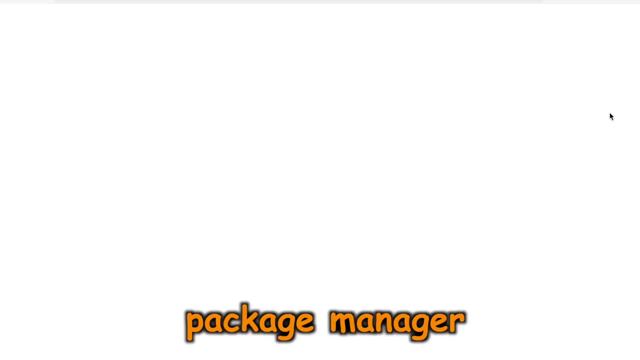 but it's actually executed on the Jupyter Notebook server. Again, you don't have to worry that much about how it works exactly, but this is just an overview. Now, to install Python and Jupyter Notebook, we're going to use something called Anaconda. Anaconda is something called a package. 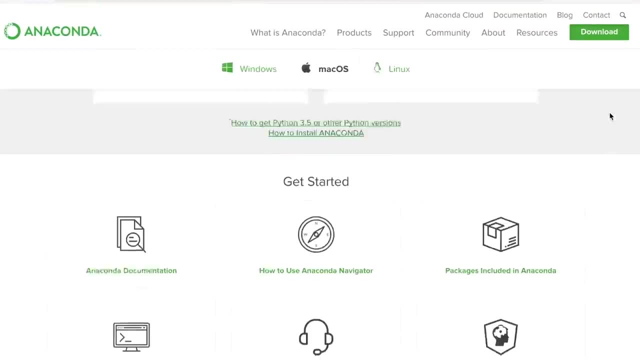 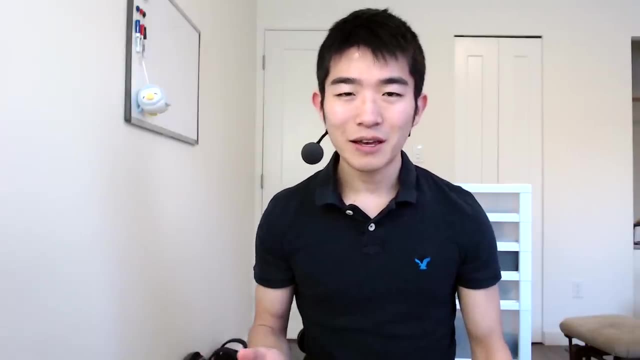 manager which allows you to install many programs at once. This particular package manager, Anaconda, is actually used for installing math and science libraries, but you don't have to worry about that. The only thing you need to know is that when you install Anaconda, it comes with 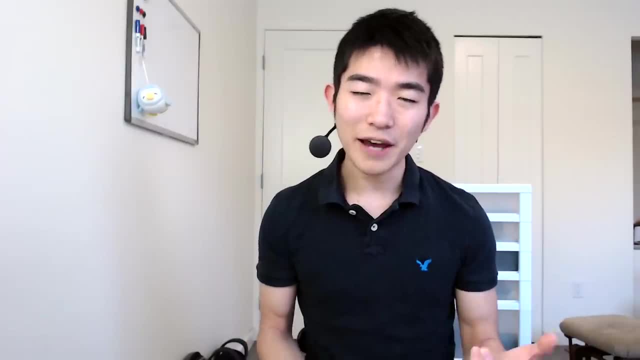 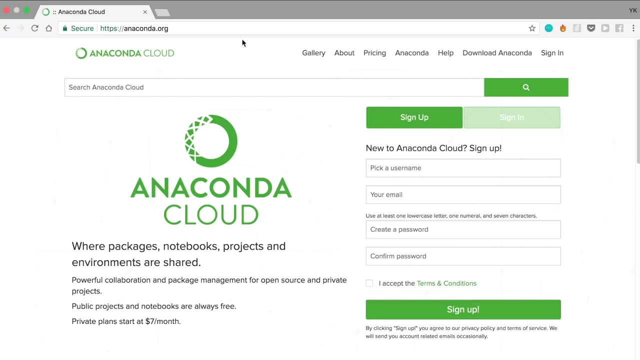 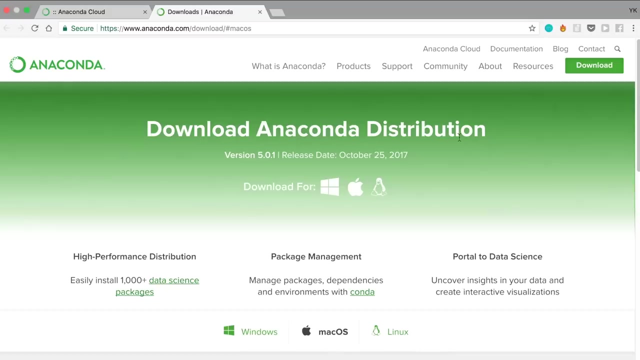 Python and Jupyter Notebook, so you don't have to install Python or Jupyter Notebook separately on your computer. Let's now install Python and Jupyter through Anaconda. Go to anacondaorg and then click Download Anaconda and select whatever platform you're using, whether it's Windows, Mac or Linux. 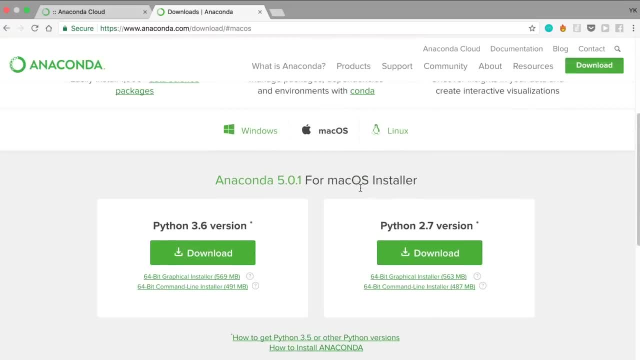 I'm using Mac here, so I'm going to click Mac OS here, and there are two options here: Python 3.something, or Python 2.something. Make sure to use Python 3.something, because we're going to use Python 3 instead of Python 2 throughout this course, So click. 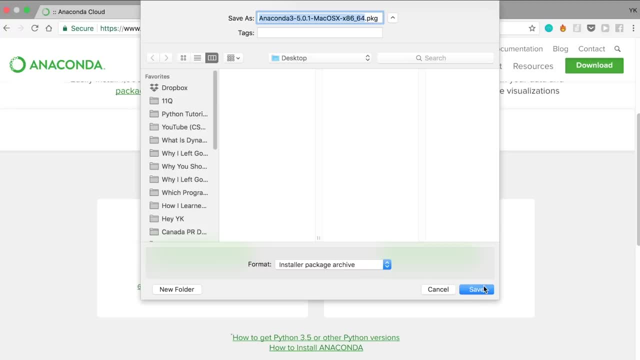 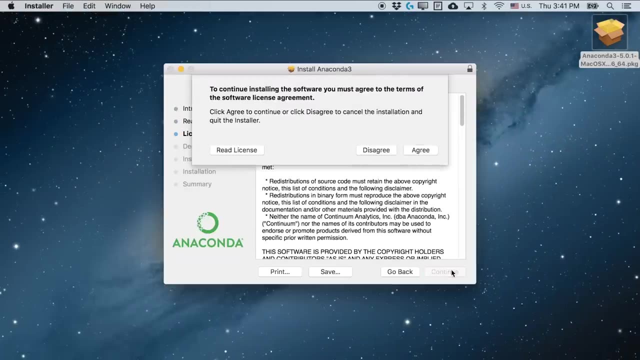 download and then save this file wherever you want to save it. Once you've saved this file, all you have to do is download it, Just open it, and then click continue, continue, continue, agree with everything and then select install for me only or install. 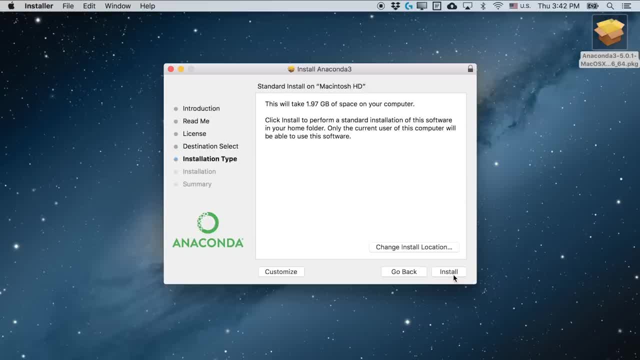 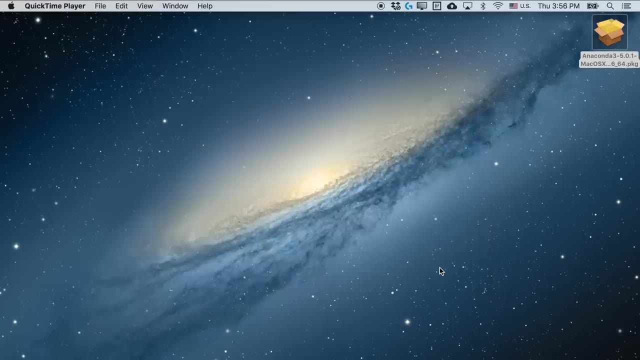 on a specific disk- It doesn't matter which one you choose- and then click install, And this process will probably take a while for you. Once this process is done, you should see something like the installation was completed successfully. Once you see that, just click close and you're. 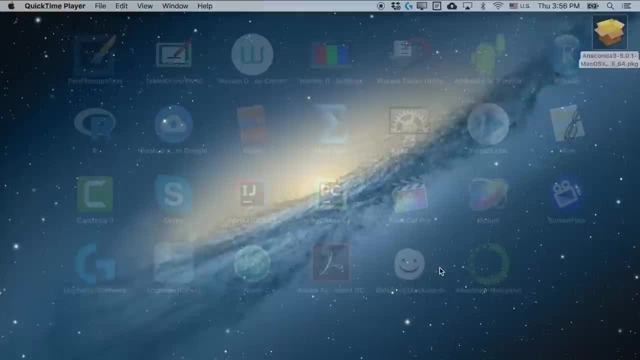 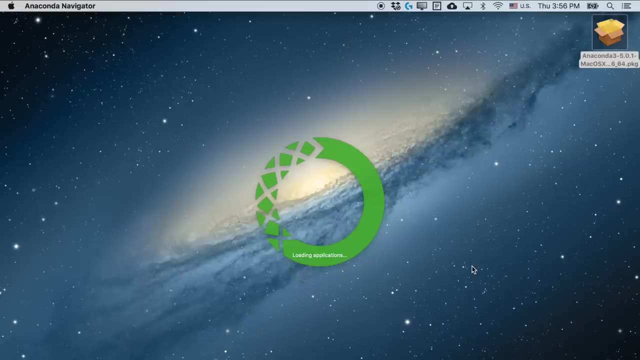 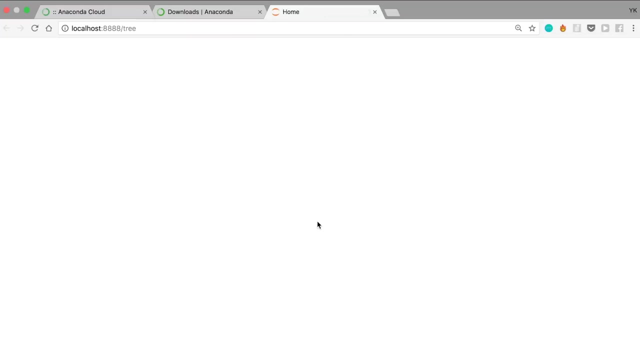 all set To launch Jupyter. you need to launch an application called Anaconda Navigator. Just launch that in the usual way. you launch any other application and then find Jupyter Notebook and click launch. Like I said before, you should see a browser tab or a window opening up. 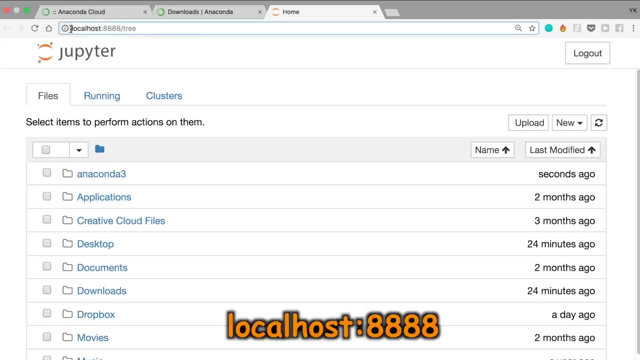 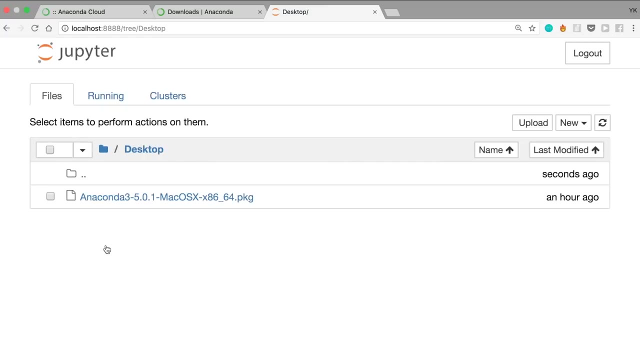 and it should be at the URL localhost, colon 8888 or something like that. Okay, let's now create our first program. First, go to whatever the folder you want to create your first program in. I'm going to go to desktop And once you click it, you can see that my current location is desktop, because 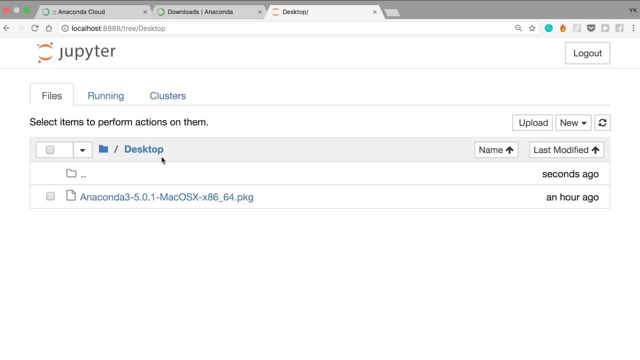 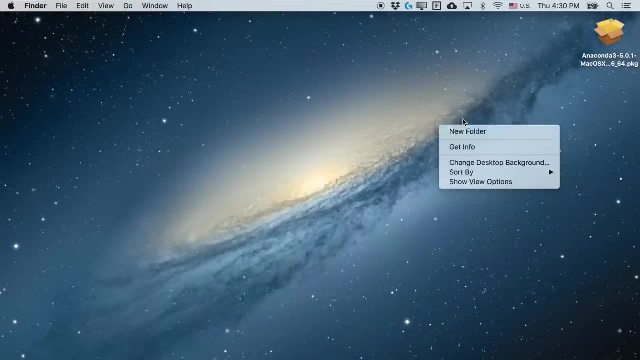 it's shown at the top right here. Before you create your first program here, I'd personally recommend that you create a new folder. So I just went to my desktop, I clicked right click and then new folder. I'm going to call this folder. 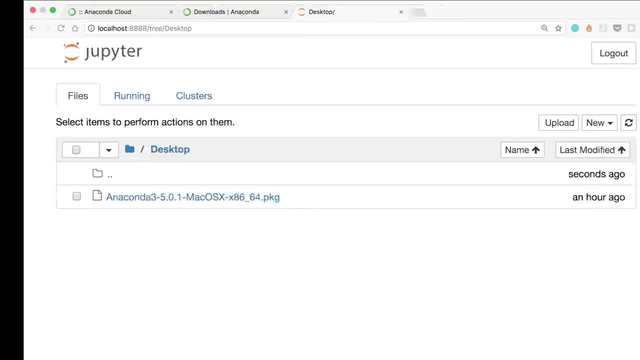 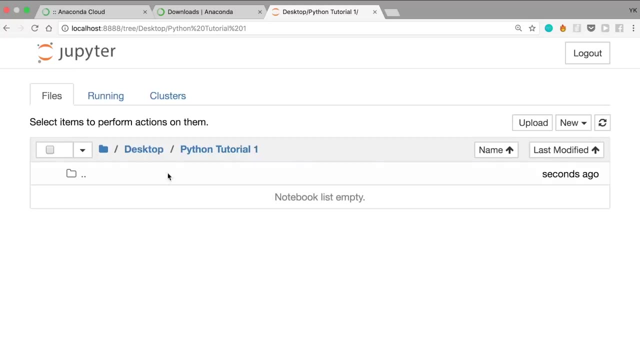 Python tutorial 1.. And once you create that folder you should see in the Jupyter Notebook interface 2, click that and you'll see that the current location is Python tutorial 1, within desktop, right here at the top, To create a new file, or a new notebook file, as they say just. 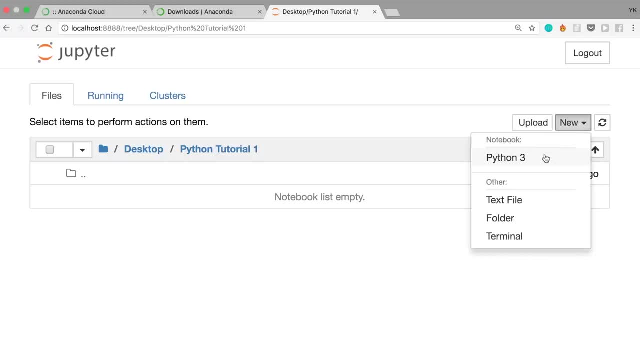 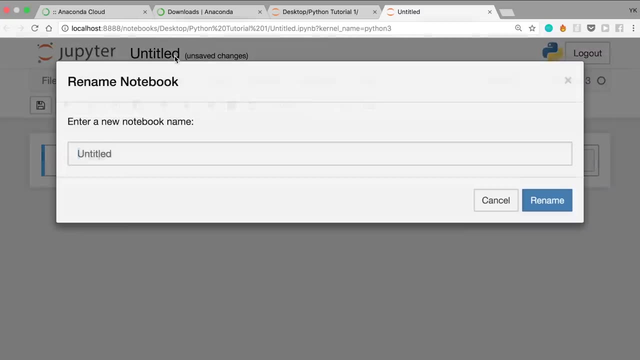 click new at the top right hand corner and then click Python 3.. So a new notebook has been created here. Change the name of the notebook to Python 3. And then click new And then click new And then change the name of this notebook from untitled to. let's say what are our variables? Click. 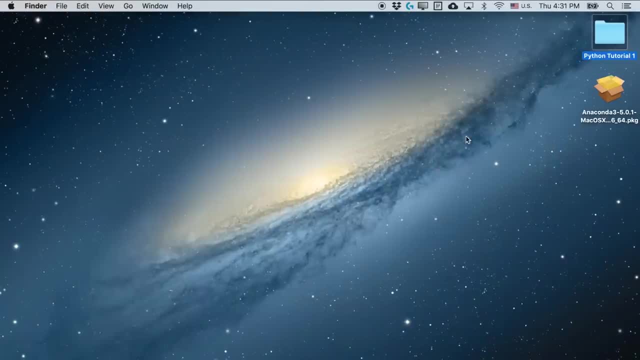 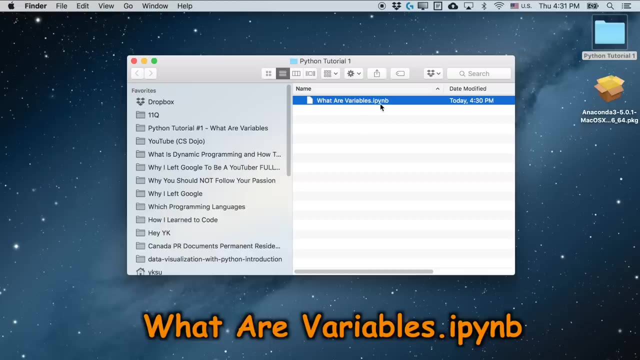 rename And once you do that, if you go back to desktop and the folder that we just created- Python, tutorial 1, you'll see a new file. what are our variablesipynb And ipynb is just an. 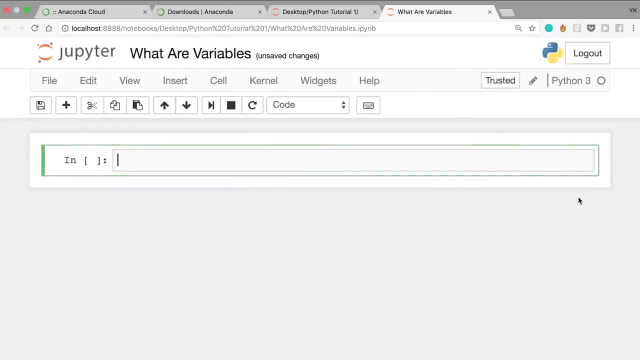 extension for Jupyter Notebook. Now in Jupyter Notebook there's something called a cell. Each cell represents a set of code and the box you're looking at is a set of code, And the box you're looking at right now is one cell. So you can type in any Python code here, For example print. 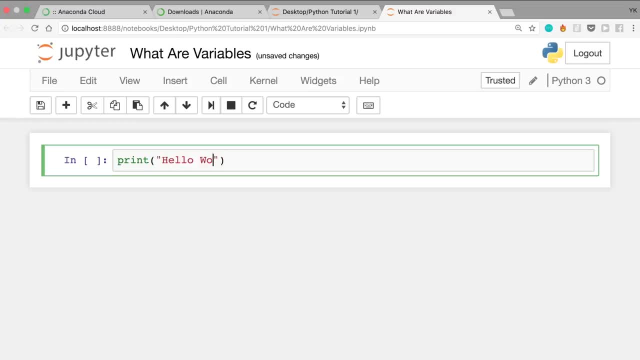 parentheses, double quotes, hello world. And when you run this cell using this button at the top, it executes all the code within the cell. So let's run this cell And you see that the string hello world is printed. So this text, hello world is something called a string. It's usually enclosed. 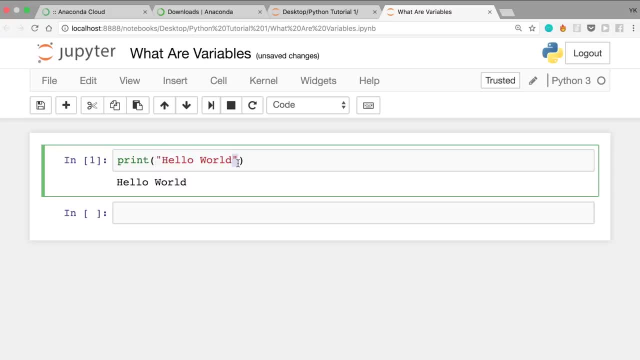 by either double quotes or double quotes, And when you run this cell it executes all the code within the cell. So this cell is printed in a single quote. So it's basically a set of characters. So, assuming that this is your first time coding in your life, I'm going to explain this line a little. 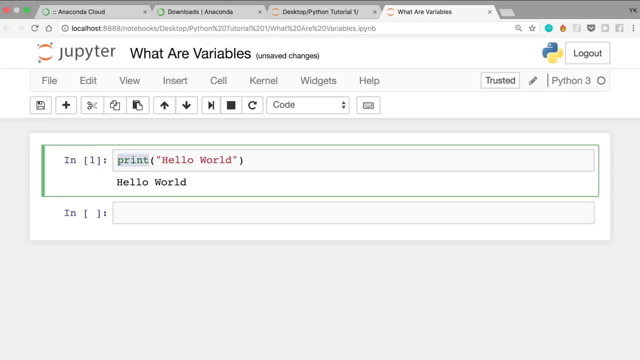 bit more carefully. So this says: print whatever's in the parentheses, these two parentheses, and that happens to be hello world, the string. And when you run it again, it's printed right below this cell: hello world. And the important thing to note here is that if you don't type in the exact 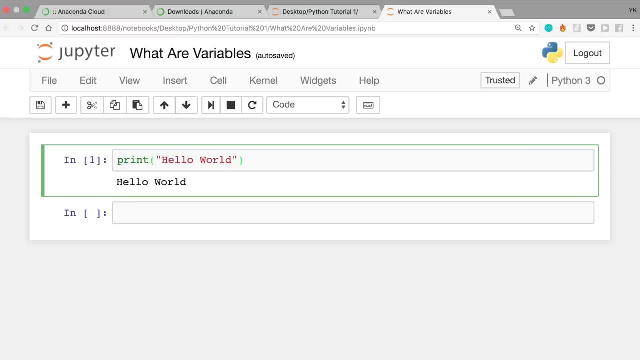 set of characters that you see on the screen. you're just going to get a string, And the important thing to note here is that if you don't type in the exact set of characters that you see on the on the screen, it might not go right. 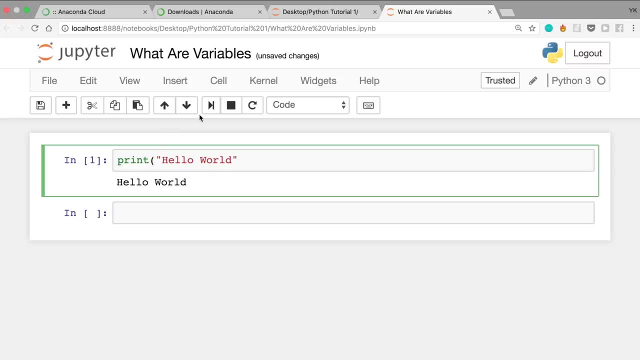 So, for example, if you forget to close the parentheses and run the cell, you'll get an error. And if you use, for example, curly brackets instead of regular parentheses, you also get an error. And if you forget to close the quotation marks. 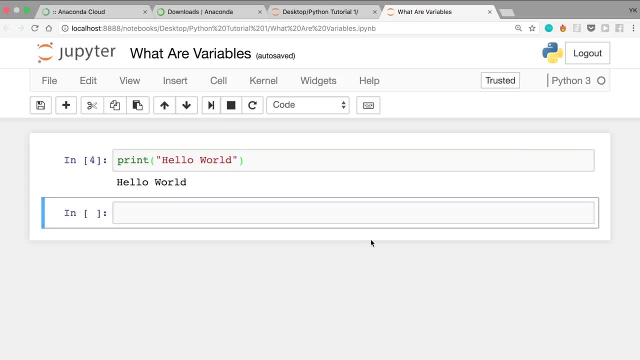 it's the same thing. So let's try using this print function a little bit more. In this cell that you see right here in the green box, you can type in print double quotes, more string, And actually, instead of using double quotes. 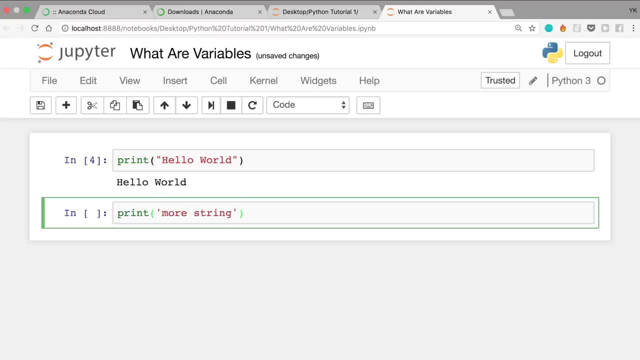 you can also use single quotes in Python and then you can run this cell and the string more string is printed. So you can use single quotes and double quotes pretty much interchangeably in Python, And then you can also print not just a string. 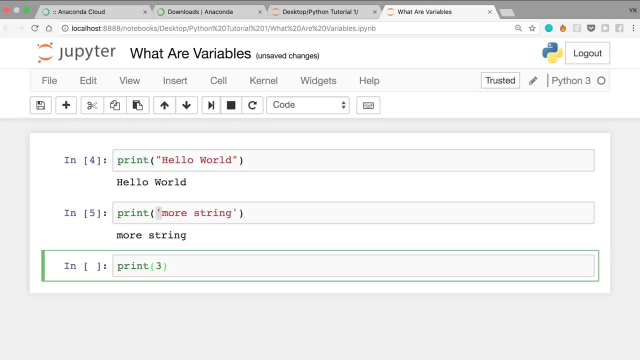 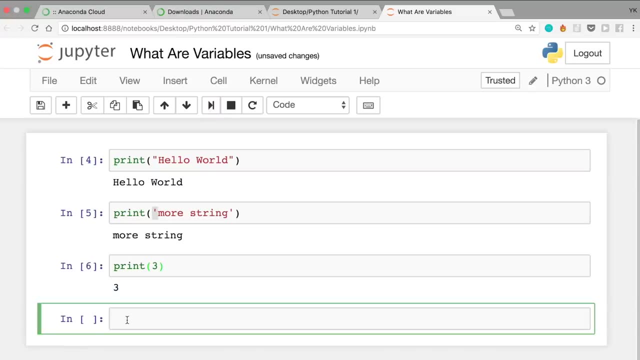 but also a number. So you can say print parentheses three and then when you run this cell, the number three is printed And you could also have multiple lines within the same cell as well. So in this cell you can write print. 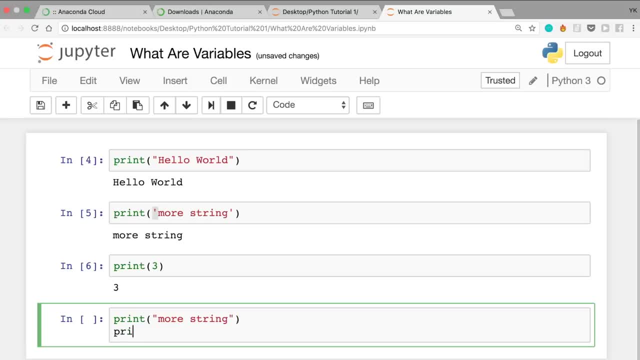 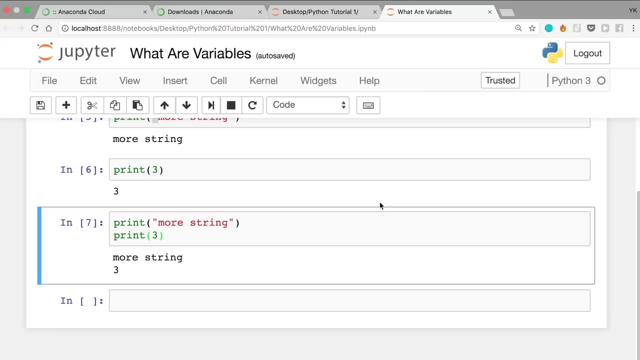 let's use double quotes here: more string and then print three. So when you run this cell, these two lines are executed one by one, So you'll see more string and three printed just one after another. So let's now dive into. 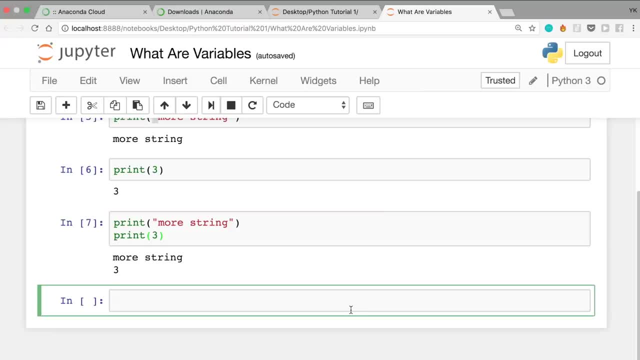 our main topic here, namely what are variables. Before I explain what are variables exactly in Python, I'm going to show you some sample code. You can write a equals one, And what this means is that assign this value one, this number, to the variable named a. 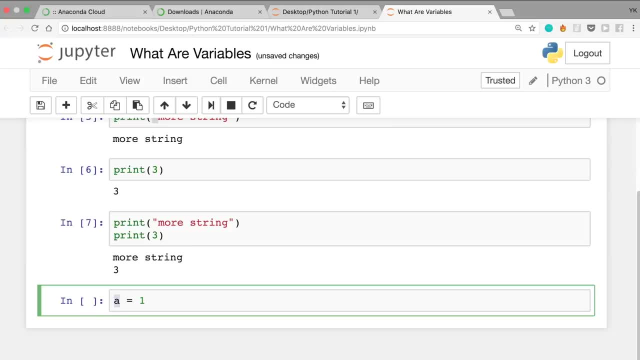 You can think of it sort of like the variable a containing the value one. That's not 100% technically accurate, as I'll explain later, but that's one way to think about it. So when you run this cell you won't see anything printed. this time. 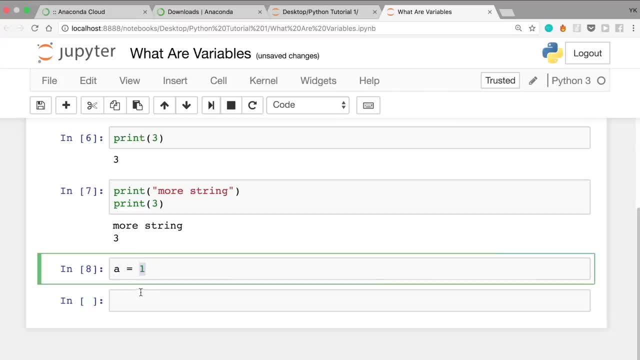 but the variable a now contains the value one, Or a more technically accurate way of thinking about it is that the variable a refers to the value one And you can check what's inside the variable a by printing the variable with print parentheses a, And note here that there are no double quotes. 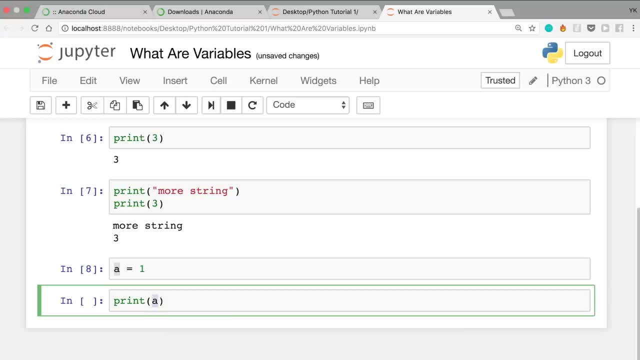 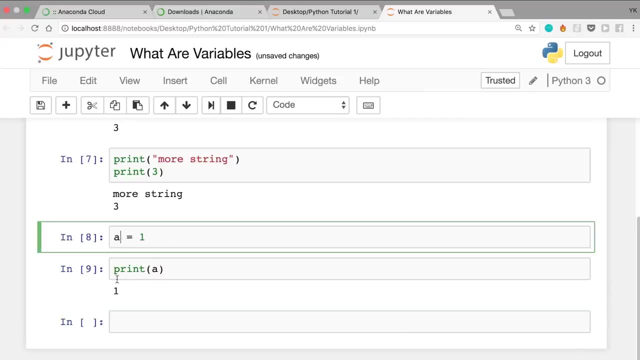 or single quotes around this character a, And that's because a is not a string, it's a variable, And when you run this cell you see the value a is referring to, which is one, And you can do the same thing with different variables. 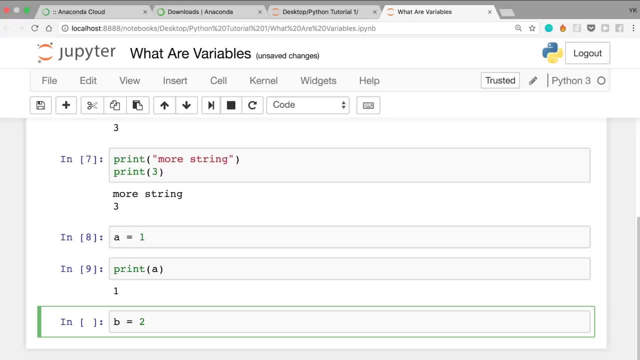 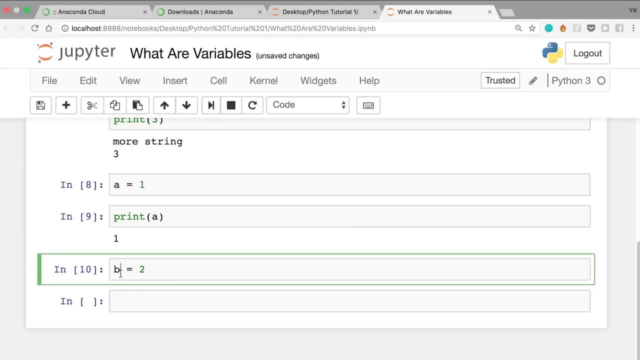 So you can write b equals two. So the convention here is you write b space and then equal space and two. This line says assign the value two to the variable b And when you run this cell again, the variable b refers to the value two. now 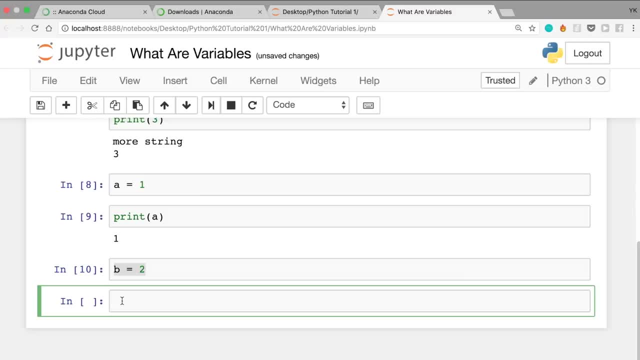 So if you haven't, for example, seen this code and if you want to know what's inside the variable or what the variable refers to, you can write just like before. print parentheses b: no single quotes or double quotes. run this cell with this button right here. 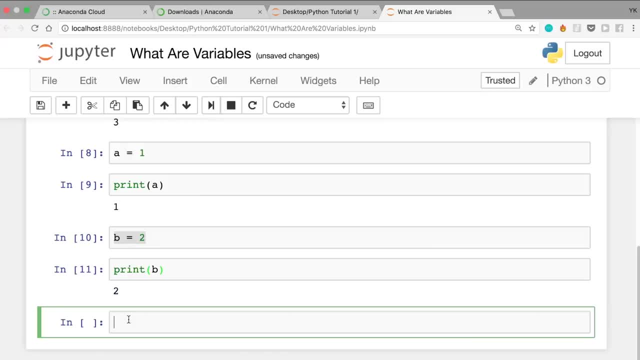 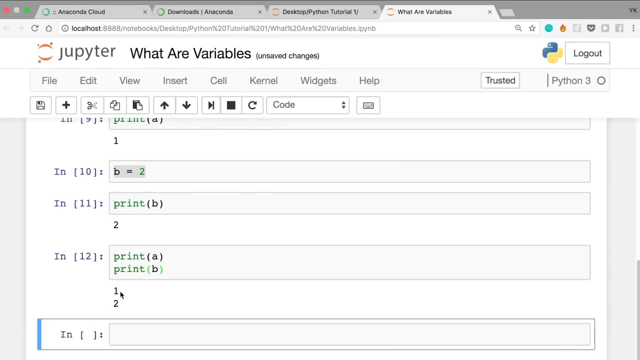 And then you'll see the value b is referring to. Just like before, we can write multiple lines within a single cell right here by writing print parentheses a, print parentheses b, And when you run this cell you'll see one and two. 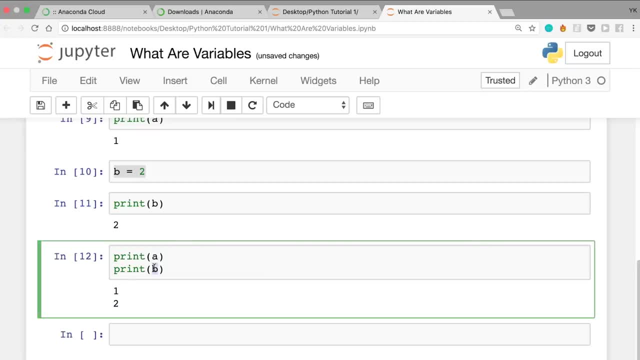 So one is what a is referring to and two is what b is referring to. So a variable doesn't necessarily refer to a number. It could refer to a string. So if you write, for example, c equals either double quotes or single quotes. 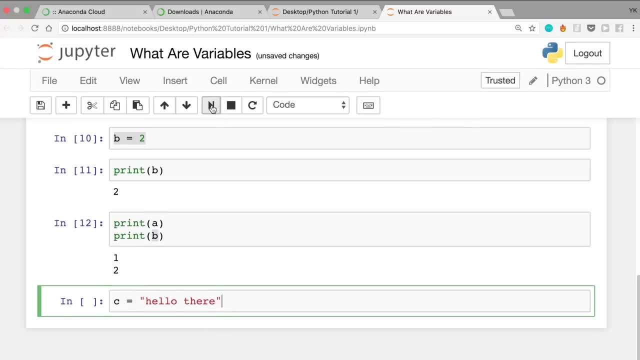 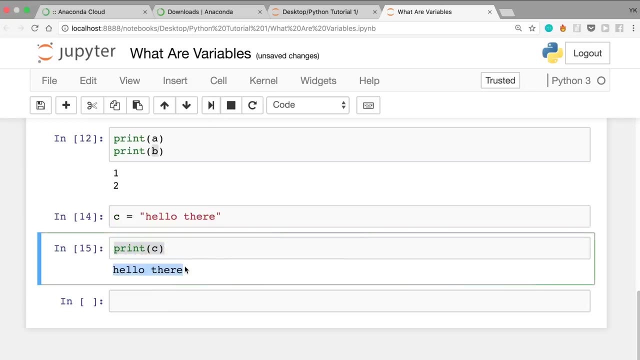 hello there And when you run this cell, c now refers to the value or the string hello there And when you print c you should see hello there printed. So I just run this cell and the string hello there has been printed. 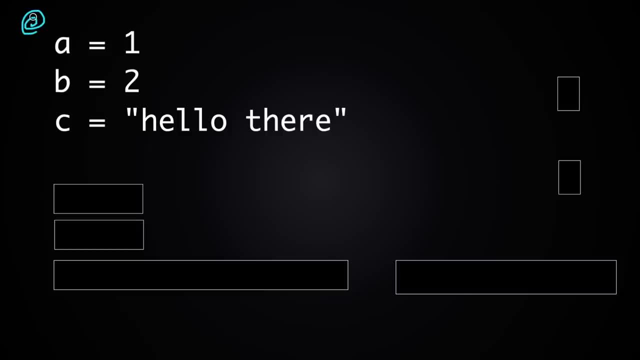 So let's now quickly talk about what variables are in Python. When you write a equals one in a different language, for example c or c plus plus, the correct way to think about it might be as a box. So you have a box a and a. 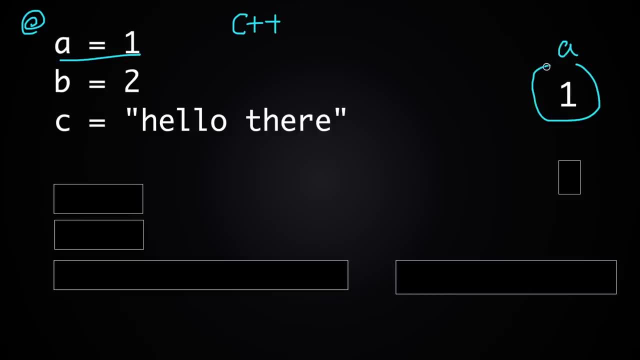 So you have a box, a, containing the value one, But in Python this is not the accurate way to think about it. The more accurate way to think about it is that a is more like a name tag, And this can refer to any value you want. 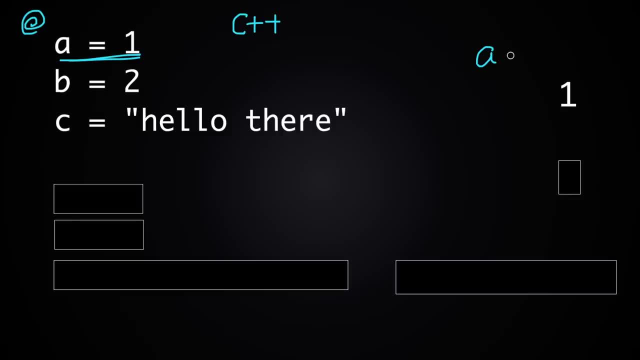 And when you say a equals one, you're saying a refers to the value one. now, These two ways of thinking about it. they might not seem that different right now, but it's going to be more important later. And in Python you can create a new variable by writing, as we saw. 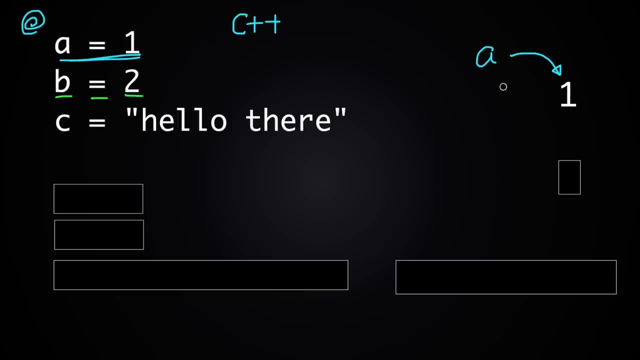 b equals two And this says the name b or the variable b now refers to the value two And, just like you saw, a variable can refer to a string as well. So if you write c equals, hello there, you're saying the variable c refers to the string. hello there. 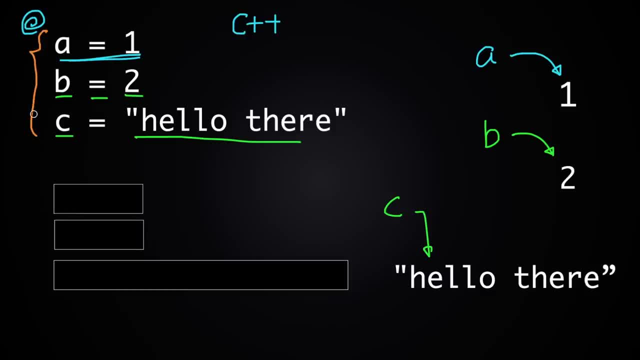 Once you master that basic concept, you'll be able to move on to a slightly more advanced topic. Let's say you run these lines of code and then you want to run more code. For example, d equals two, Then what happens is the variable d, of course. 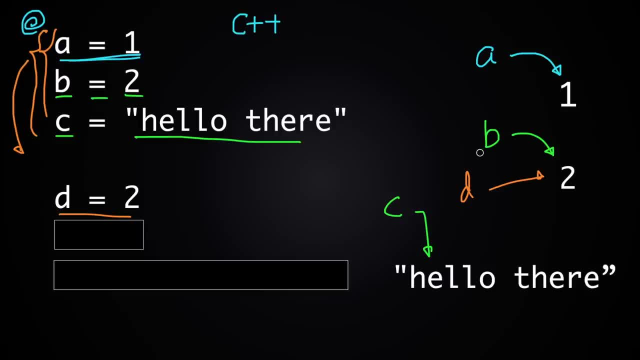 refers to the value two, which the variable b also refers to. So it's totally possible for two or more variables in Python to point to the same value, in this case two, And then it's also possible for you to reassign an existing variable to another value. 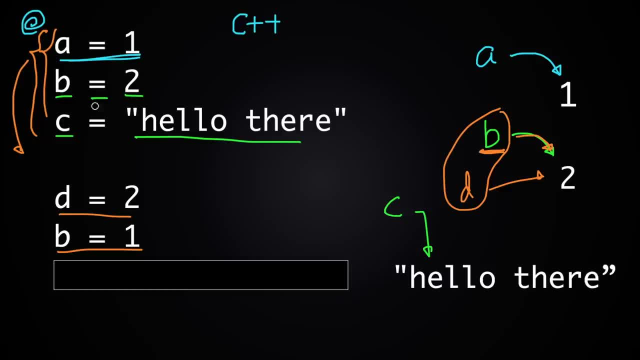 So if you write b equals one, one after executing this line of code, b equals two. after this line, b refers to two, of course, but after writing b equals one, b refers to one, which a also refers to, And you can even reassign an existing variable. 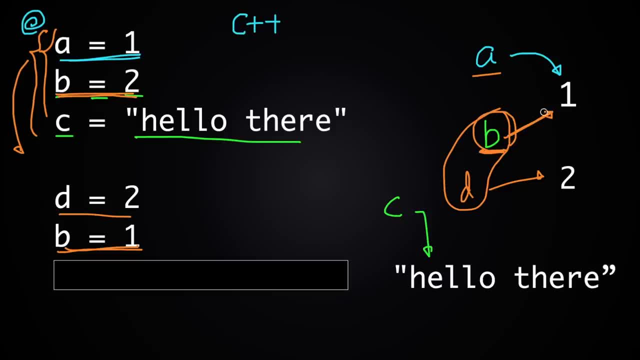 For example b, which once referred to a number one, right here to something else, for example a string. So if you write, for example, b equals double quotes, our the string. the variable b now refers to the string. ah, so let's see how this actually works out in. 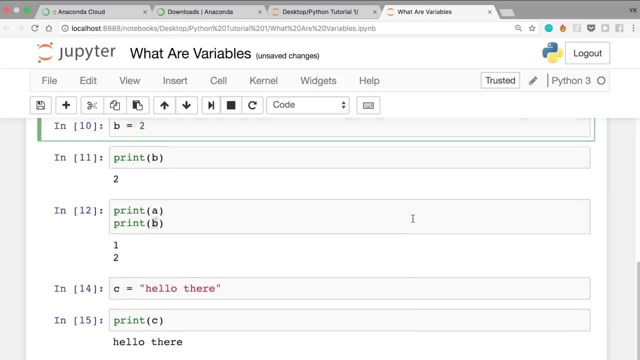 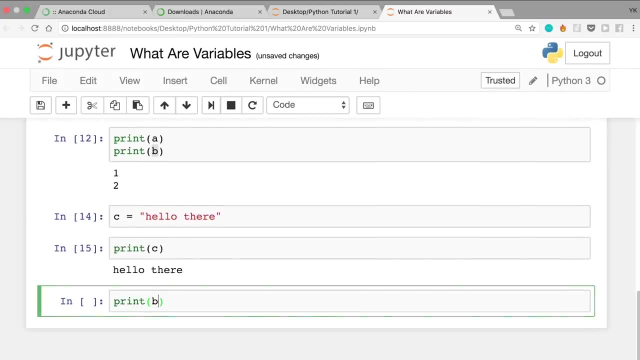 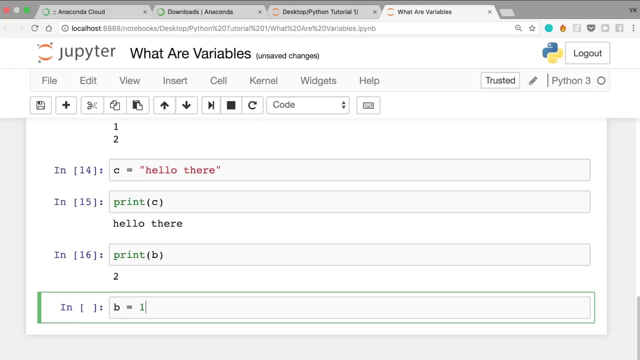 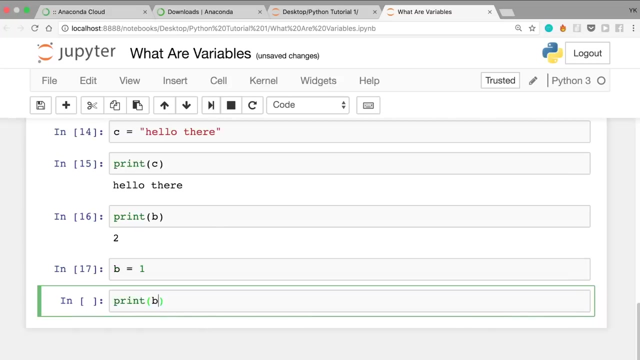 code. okay, we're going to continue on the code we had earlier. earlier we had b equals 2, so if you print b, the variable, we get the value 2, and you can reassign this variable to another value, for example 1, by writing b equals 1 and then when you run the cell and print b again, you get 1 printed. 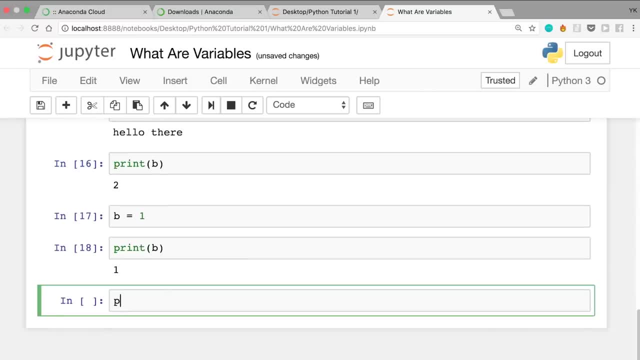 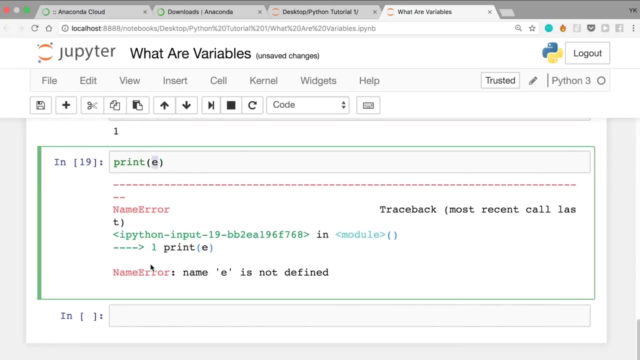 the new value and what happens if you try to print a variable that doesn't exist yet. so if you try to print- print parenthesis a, what happens? let's run the cell and see what happens. it'll actually give you an error because e doesn't exist yet and the error says name: error: name: e is not. 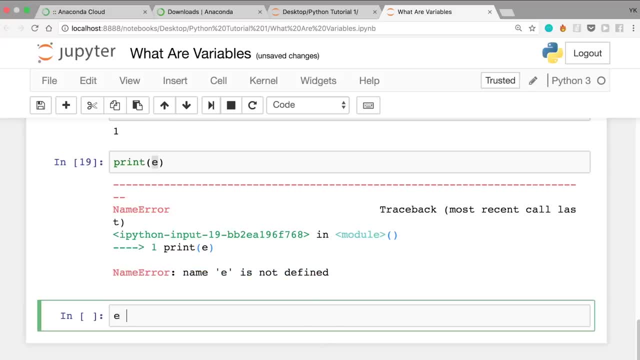 different. so if you try to print a variable that doesn't exist yet, it'll actually give you an error because e doesn't exist yet. so if you try to print a variable that doesn't exist yet, so if you find yet, so that makes sense. let's fix that by writing: e equals- this is a string, and this way: 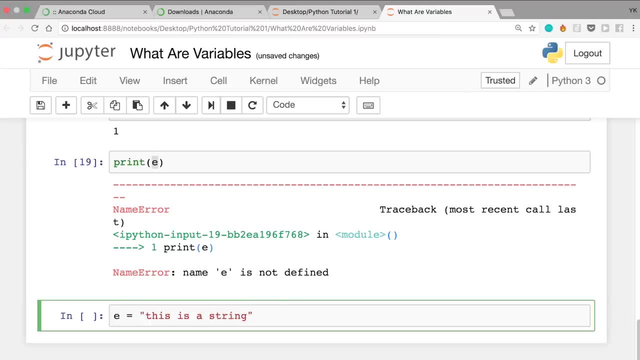 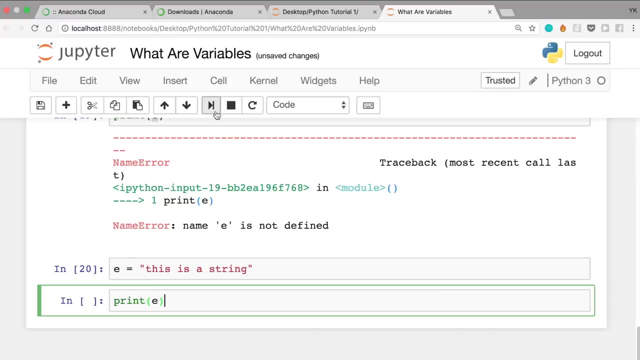 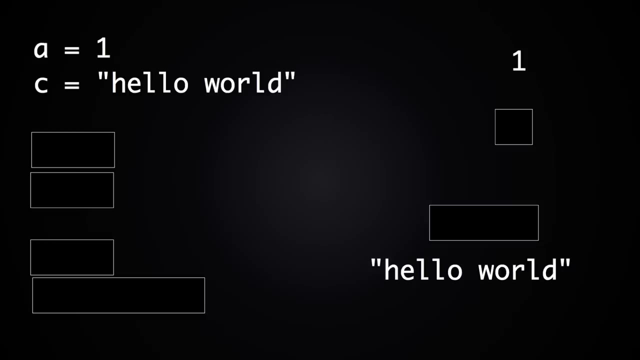 the value- this is a string- is assigned to the variable e and the variable e exists in the system. so if you print e with print parenthesis e and when you run this cell, you don't get the error anymore. and let's address another question you might have here. is it possible for us to 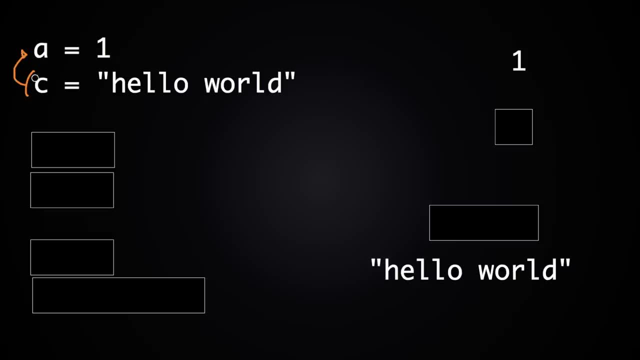 assign a variable to a variable that doesn't exist yet. so if you print e with print parenthesis e, then you're理. so if you try to print a variable, than once you score an ansf. another type of error, Carl yours. report it again with an example. relative to the value of the. 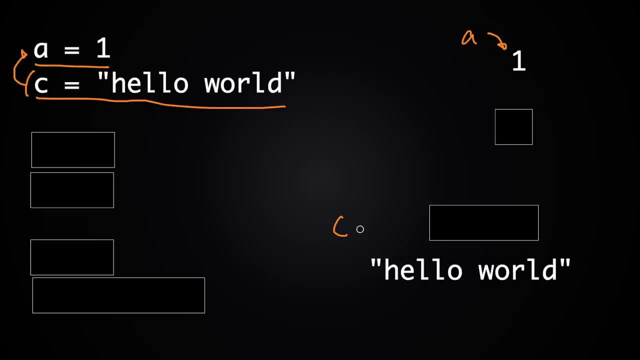 variable dp to the value of the variable dpCable, something like that. so if you write a, it will say hello world. for reference: hello world. so if you point to another one, the answer is yes. so here, if you write a equals one, A of course refers to one, and then C equals hello world, C refers to. 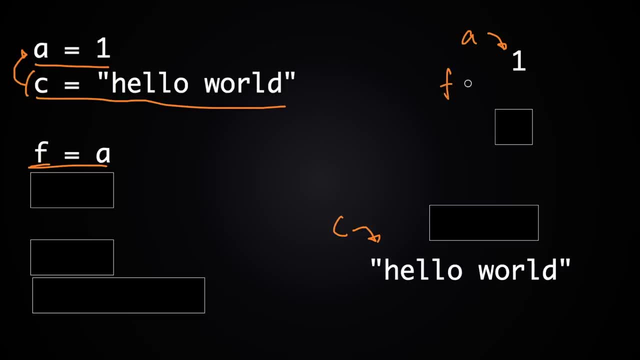 hello world. and what happens if you write F equals a. what happens then is this means the variable f, the name f refers to the value A is referring to, so F refers to one now and then when you enter. And so f doesn't refer to the variable a. instead, it refers to the value a is referring. 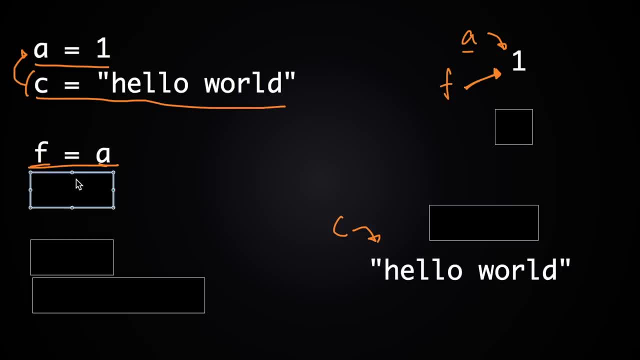 to, And this is important, for example, when you do a equals 2.. If you write that a now refers to the value 2 instead of 1, but f stays at the value 1. And this might not be the case if f was referring to the variable a. 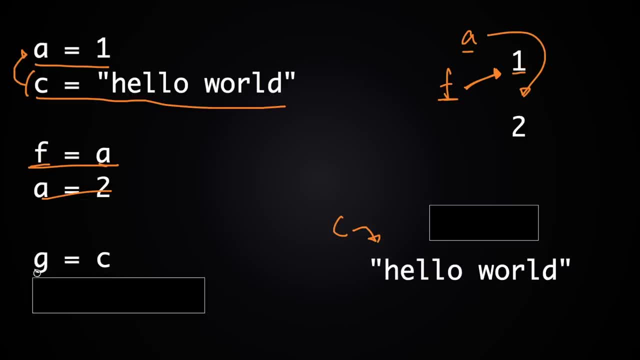 Let's take a look at another example here. If you write g equals c, the variable g will refer to whatever the value c refers to, which is hello world. And then, once you write c equals hello, c will refer to the new value hello, right here. 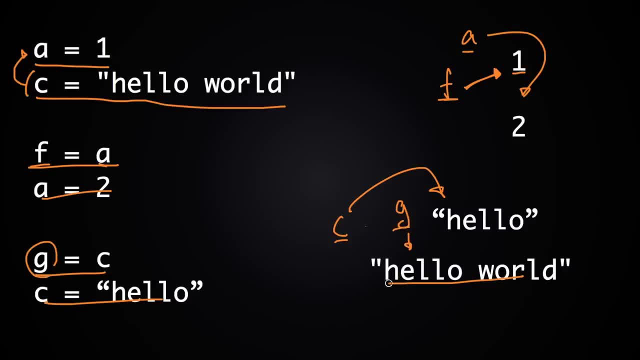 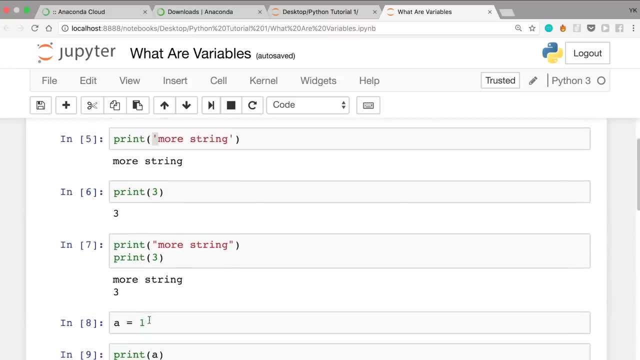 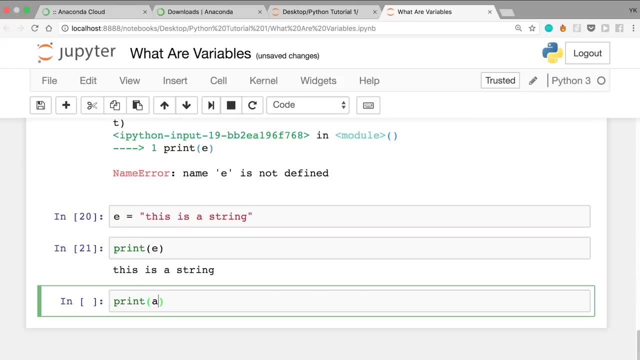 but the variable g will stay at the value hello world. Okay, let's go back into the demo. Earlier in the demo we had a equals 2., A equals 1. And then c equals hello there. So once we print a and c with print parentheses a and print parentheses c, we should see one. 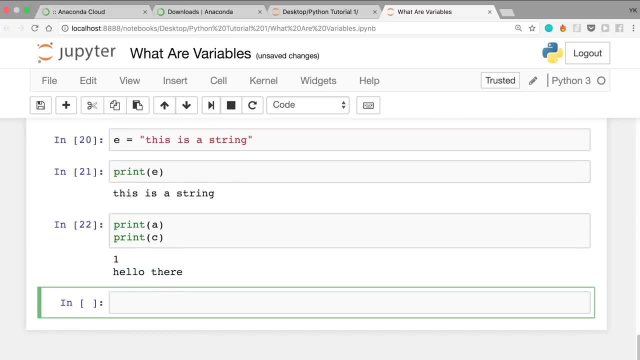 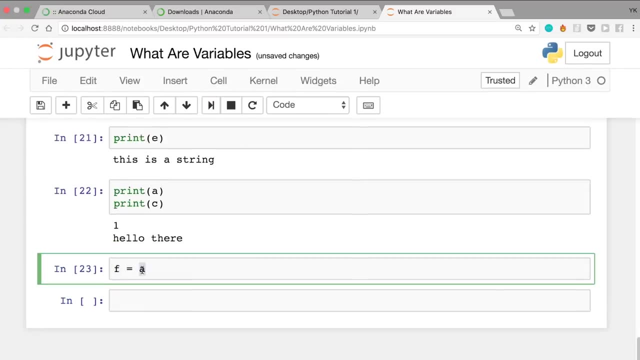 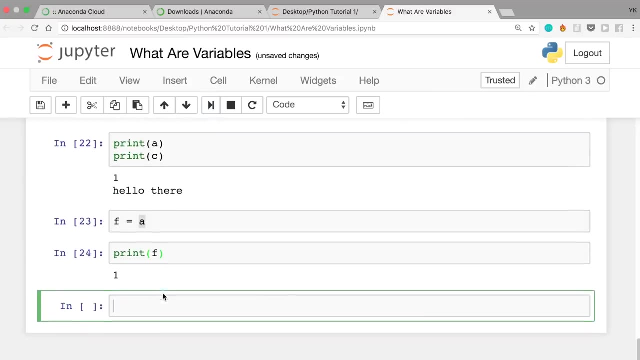 for a and hello there, for c. What happens if we write f equals a? f should now refer to whatever a refers to. So if we print f, we should see the number 1.. Okay, The number 1 printed. And what happens if we assign a to 2?? 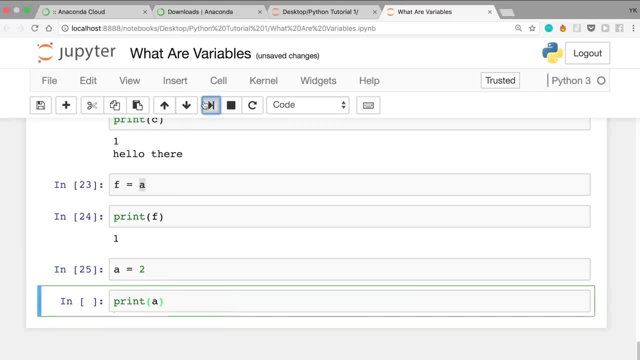 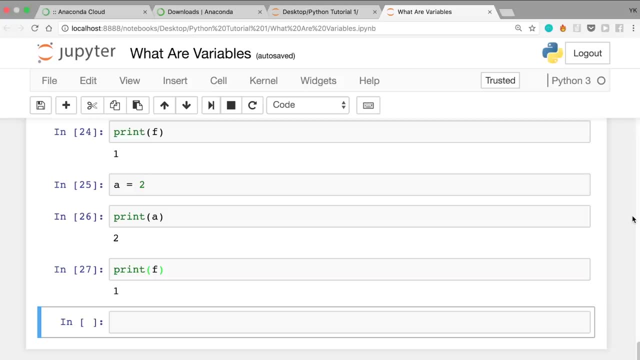 Then the value of a should now be 2, and then the value of f should stay, as I said earlier, at 1.. Okay, now I'm going to give you a quick practice problem to work on in order to solidify your 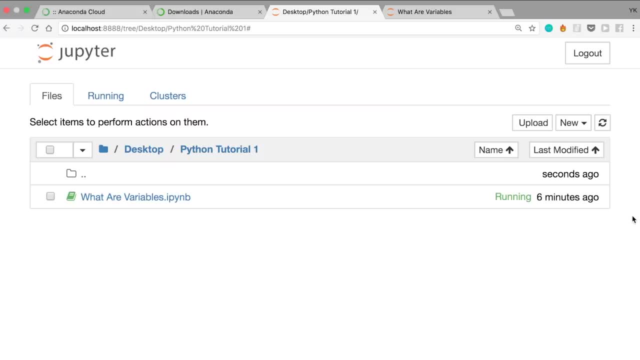 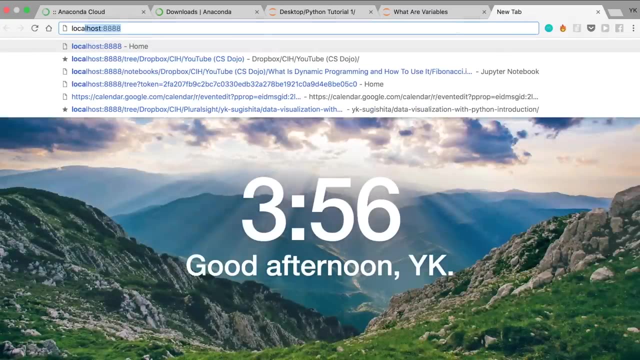 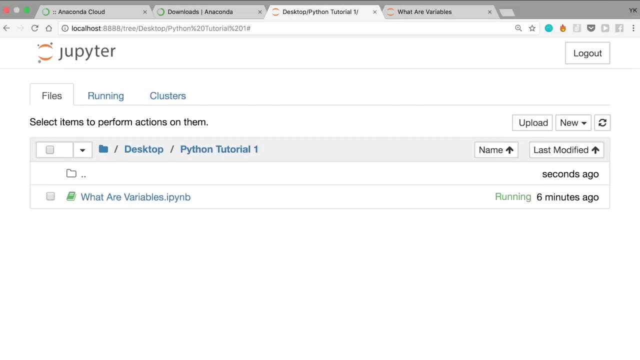 understanding of variables. And to do that go back to the previous tab of Jupyter Notebook, the navigation menu, And if you already closed that tab, Just open localhost colon 8888, or just relaunch Jupyter Notebook And then go back to the same folder as before. 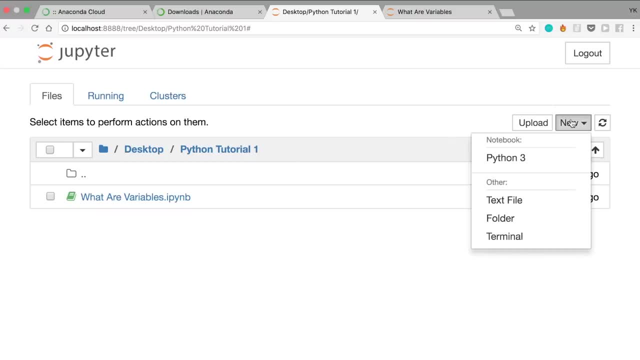 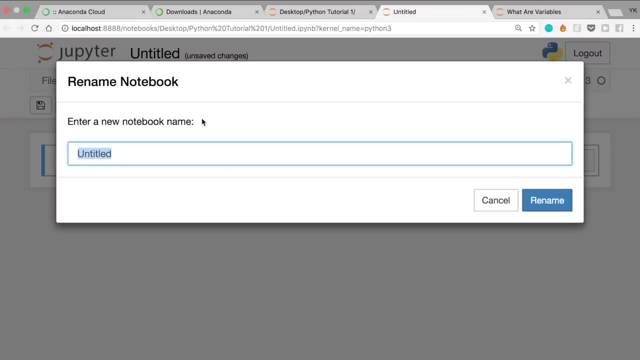 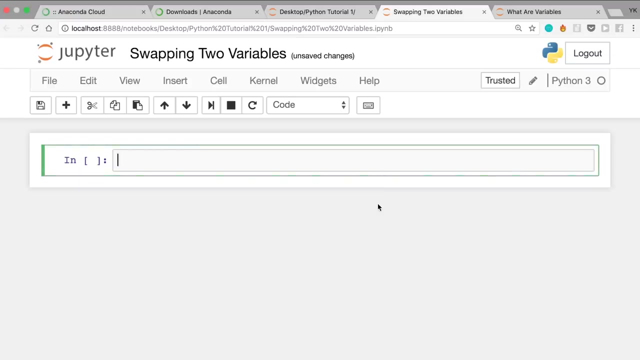 We had Python tutorial 1. Click new in the top right corner, Click Python 3 again And let's rename this notebook by clicking untitled and by changing it to swapping to variables. And here's the problem: You're given two variables. 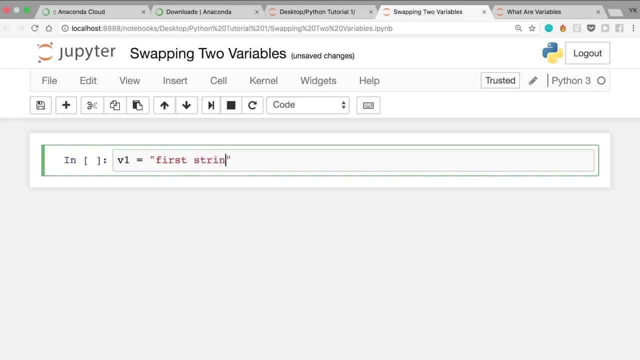 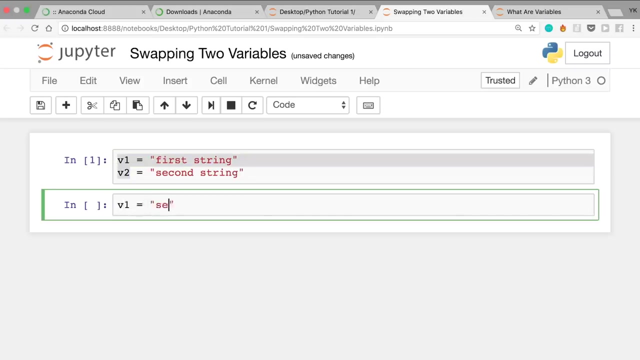 Let's say v1 equals first string in double quotes and v2 equals second string, again in double quotes. How can you swap the values within these two variables with each other? The easiest way to solve this problem is just to write v1 equals second string and then. 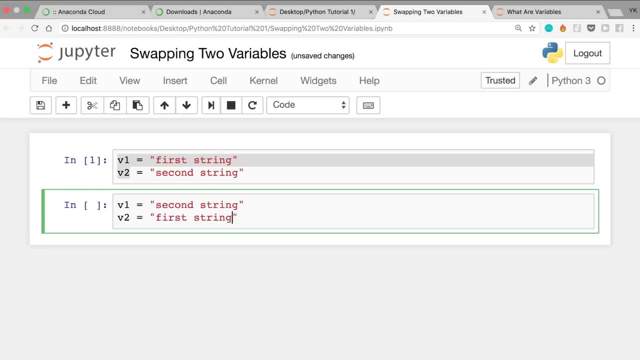 v2 equals first string. But this might not be the best solution, because if you had a much longer string it would be kind of cumbersome To repeat And then if one of the strings changes, So if first string becomes first two strings, then you need to rewrite your code right here. 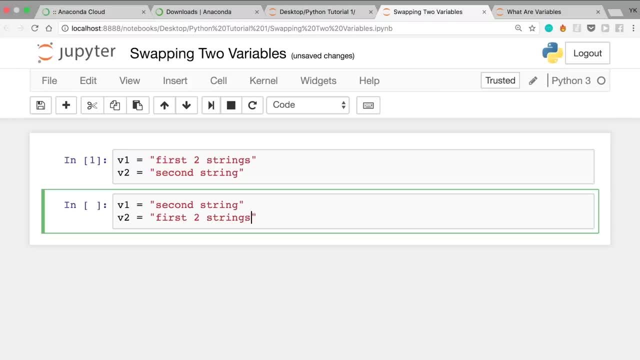 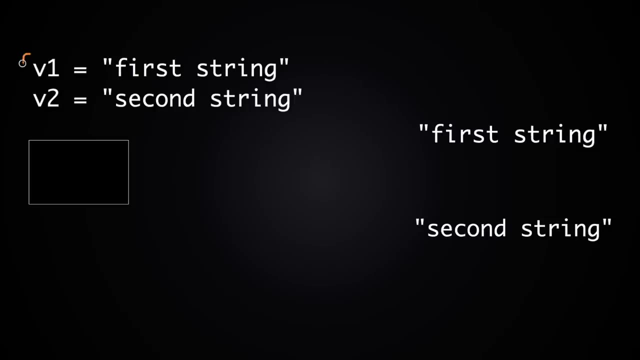 to match that, to write first two strings again. So ideally you want to be able to solve this problem without repeating the strings. Think about it for a second and then I'm going to show you what a good solution might look like. When you see this problem you might say, well, it's actually pretty simple. 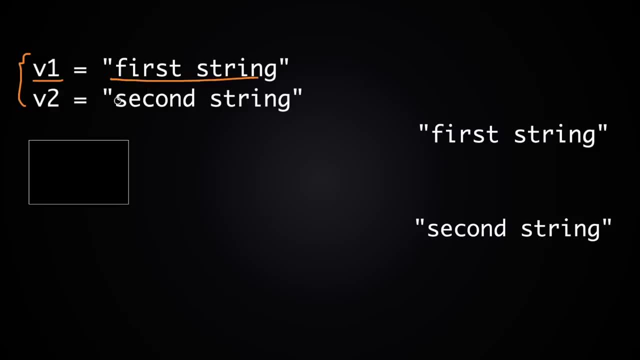 Once we have v1. Equal to first string and v2 equal to second string, So that's v1 referring to this string and v2 referring to this string. We can just write v1 equals v2 and then v2 equals v1 and we're done. 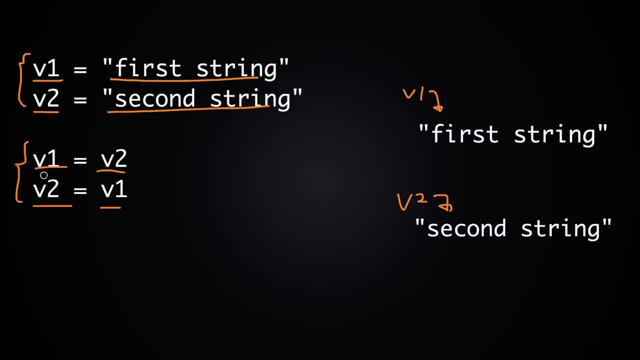 But actually this solution is wrong, because when we execute this line, v1 equals v2, v1 now refers to whatever v2 refers to, of course, which is second string. And then when we write v2 equals v1,, v2 will now refer to what v1 refers to now, which. 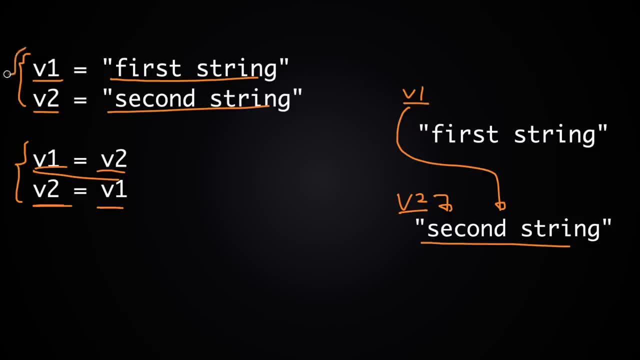 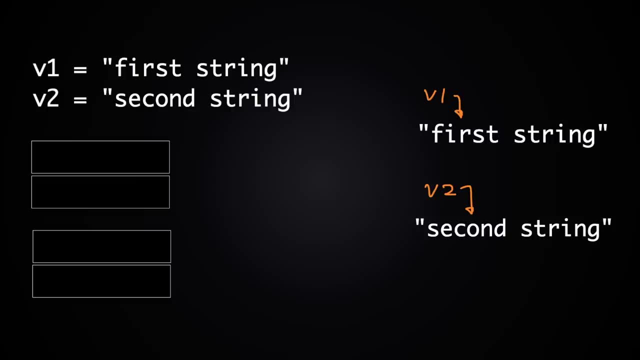 is second string. So at the end of these lines of code we'll have v1 and v2, both referring to second string, which is not what we want. Let's now see what a good solution might look like. I'm going to give you a few different options here. 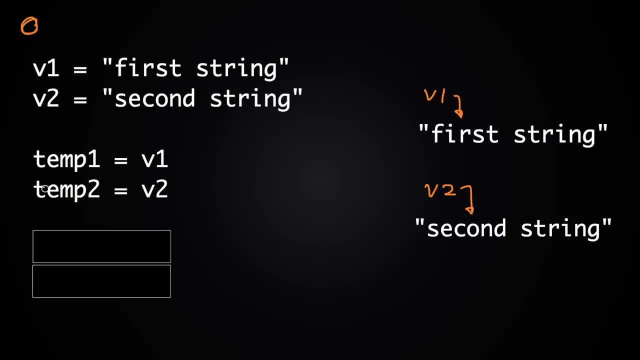 The first option is to use two temporary variables. We're going to call them temp1 and temp2.. So we're going to call them temp1 and temp2.. So temp1 will be equal to what v1 refers to. so that's first string. 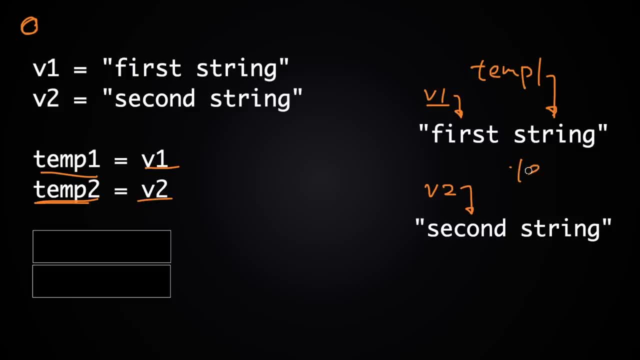 And then temp2 will be equal to what v2 refers to, which is, of course, second string, And then we'll just need to swap them together. So v1 will be equal to temp2, which refers to second string. So v1 will now refer to second string, after this line right here. 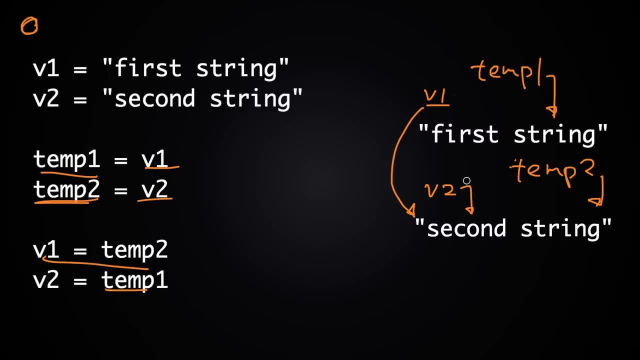 And then v2 will be equal to temp1. Which is of course first string. So v2 will refer to first string after these lines. So this is one potential solution, But actually we don't have to use two temporary variables. 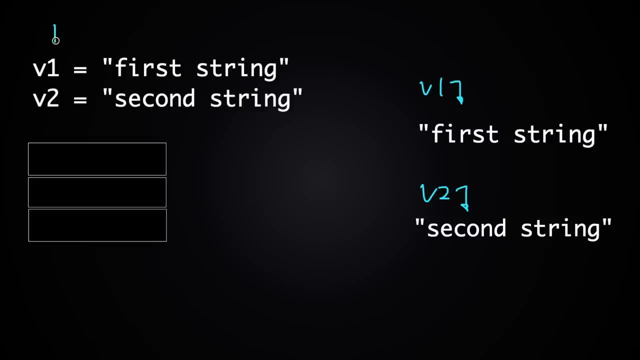 Okay, here's a solution that only uses one temporary variable instead of two. The first thing we're going to do is we're going to set a new temporary variable called temp to what v1 refers to. So temp will be v1.. So temp will be v2..